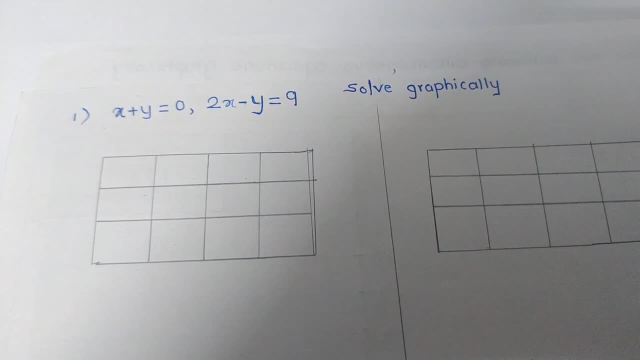 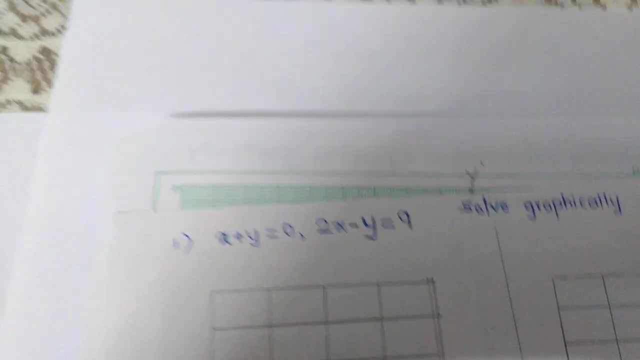 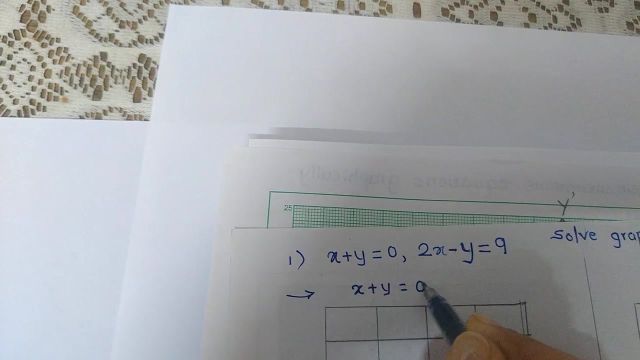 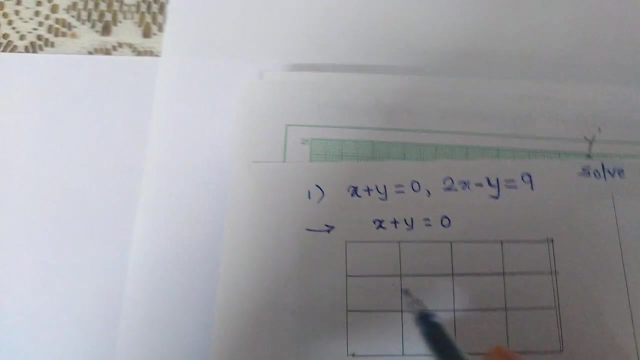 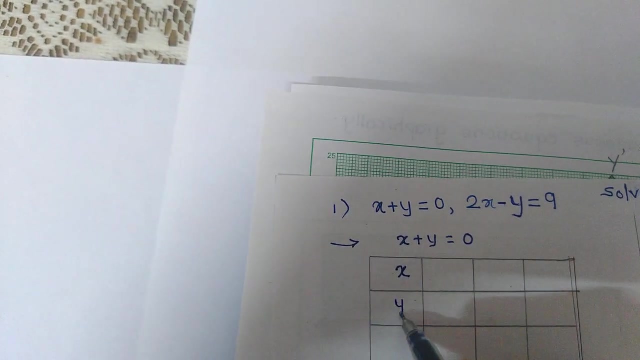 In this video we will see how to solve given simultaneous equation. graphically, Two equations are given to us In solution. consider first equation, which is x plus y, equal to 0.. After writing equation, prepare a table with four columns. In first column, to the rows you can give the headings x, y and last row can be labeled as x- y. 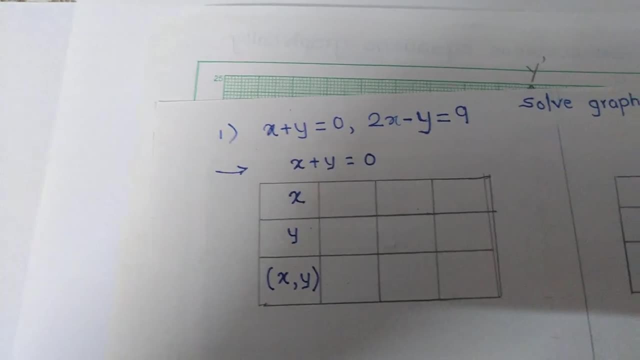 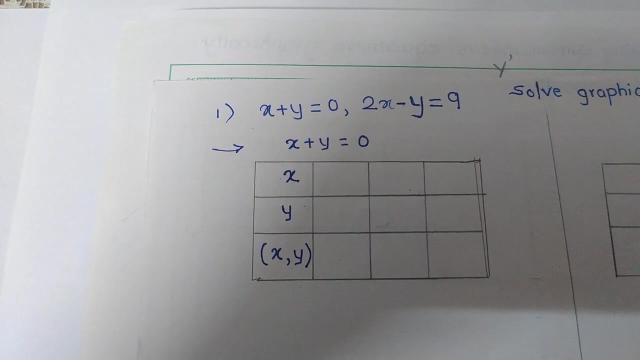 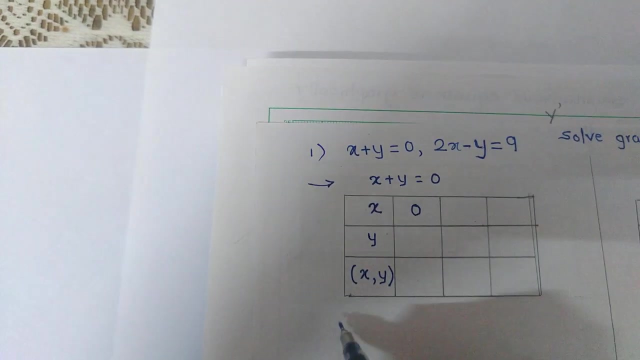 Here now consider value of x. by your mind, Any value can be considered. You can take positive value, negative value or 0. And value of y will be obtained by calculation. Suppose I consider x equal to 0. I take value of x as 0.. 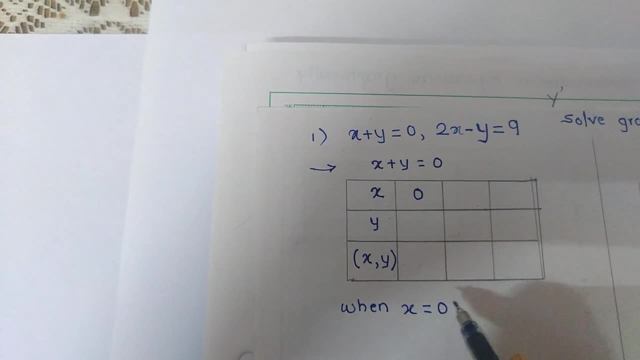 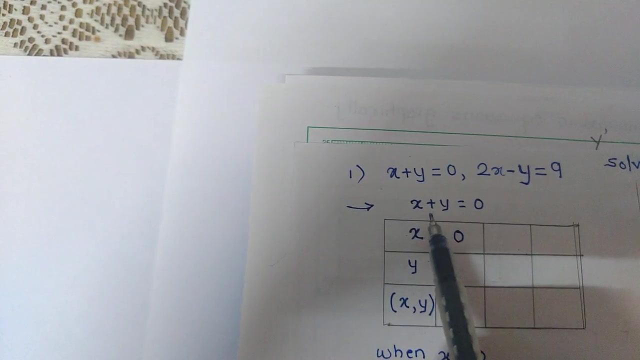 So when x is 0, we have to calculate value of y. Therefore, 0 plus y is equal to 0.. So what I have done: in first equation, in place of x I have written 0, as I considered value of x 0. 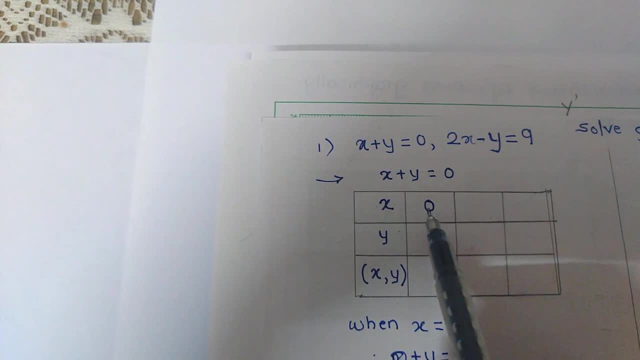 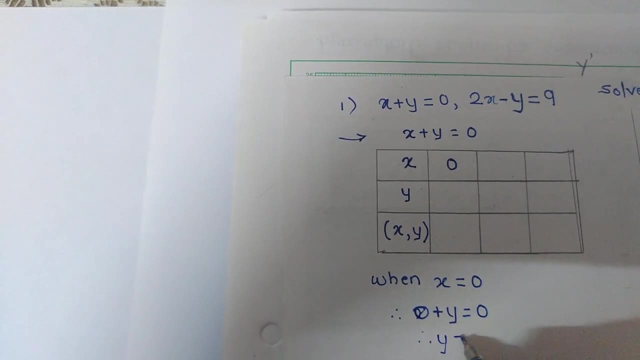 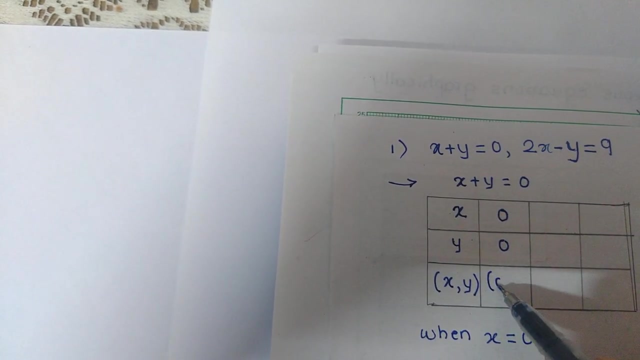 This value you can consider any number may be positive number, negative number Or it can be 0.. So in place of x I wrote 0.. 0 plus y is 0. Therefore y is equal to 0. That is, when you take x equal to 0, y is 0. So the coordinates are 0, 0.. x coordinate and y coordinate. 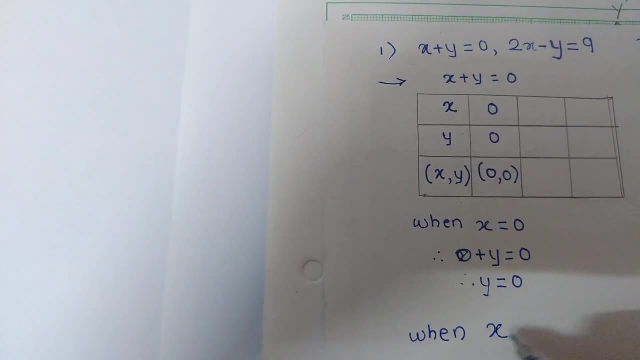 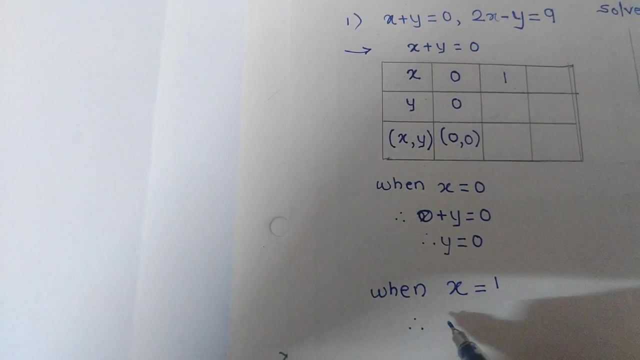 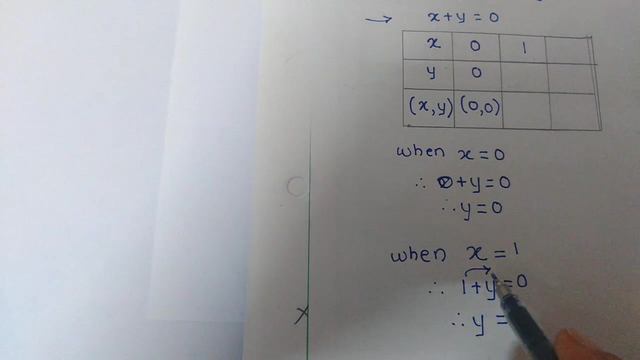 Next, consider one more value of x by your mind. Suppose now I take x equal to 1.. So when x is equal to 1, we have to calculate value of x. So 1 plus y is equal to 0. So therefore y is equal to 1 will be transferred on other side of equal to. 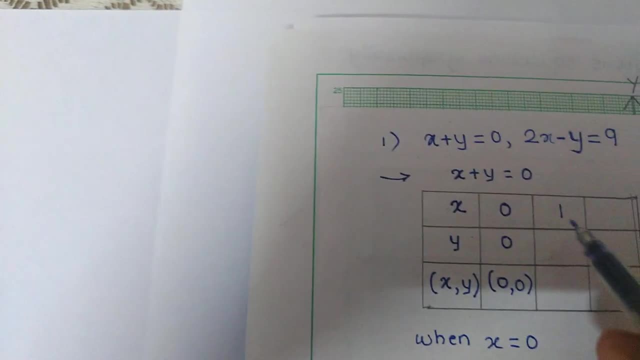 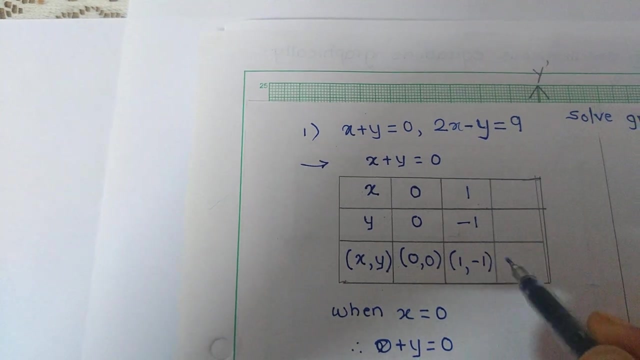 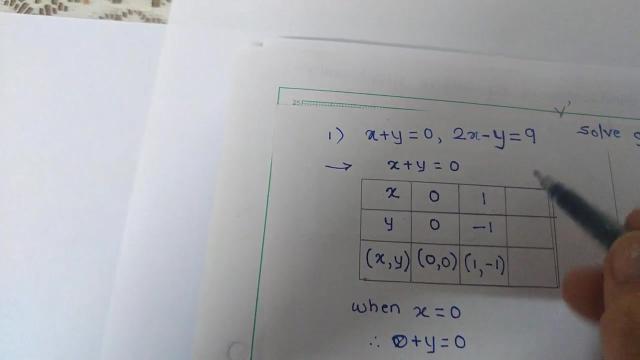 Its sign will change: y will become minus 1.. That is when x is 1, y is minus 1.. So the point is 1 minus 1.. Similarly now consider third value for x. When x is equal to suppose I take now x is equal to 2.. 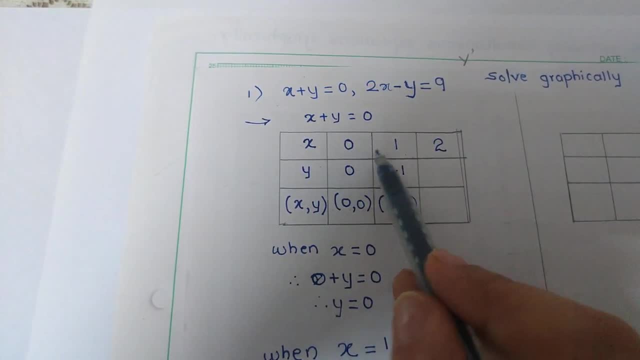 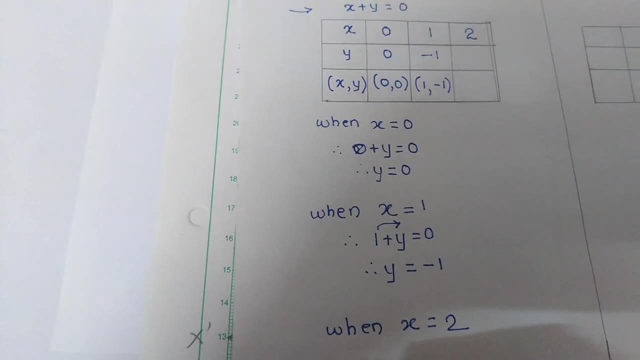 I repeat, you can consider values. So, when x is equal to 1, y is 0. Therefore, y is equal to 0. So, therefore, y is equal to 1.. You can take any values of x. So now, as I took x equal to 2, I will calculate value of y. 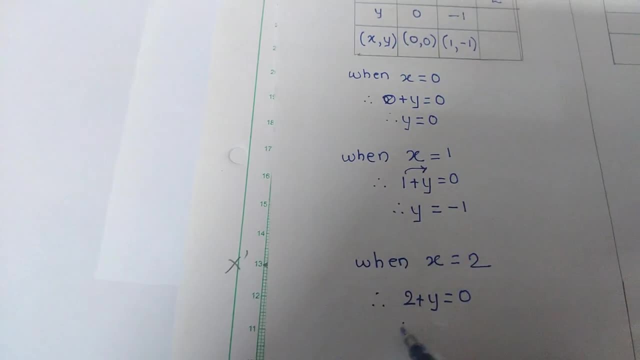 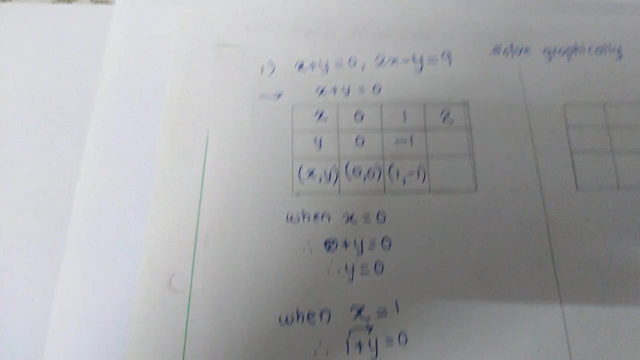 Therefore, 2 plus y is equal to 0.. So therefore, y is equal to. 2 will be transferred on other side of equal to, Its sign will change: 2 will become minus 2.. That is when x is 2, y is minus 2.. 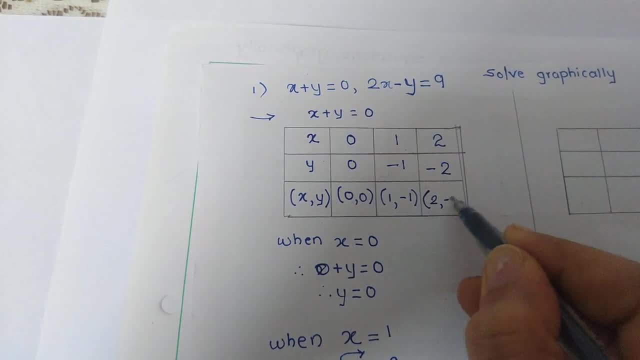 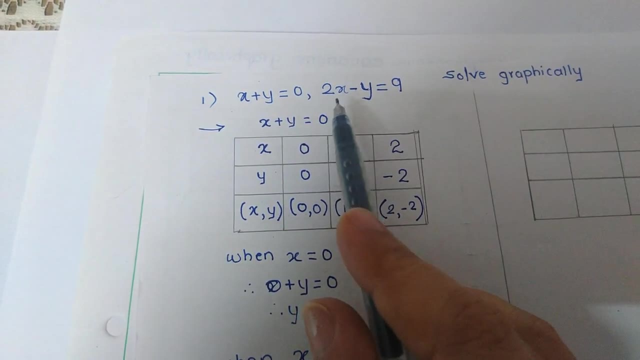 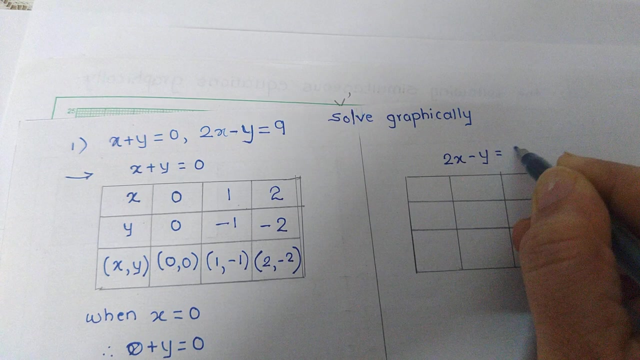 So the coordinates of point are 2 and minus 2.. This we have done for first equation. Now consider the second equation which is given in the question: 2x minus y, equal to 9.. So I write it here: 2x minus y is equal to 9.. 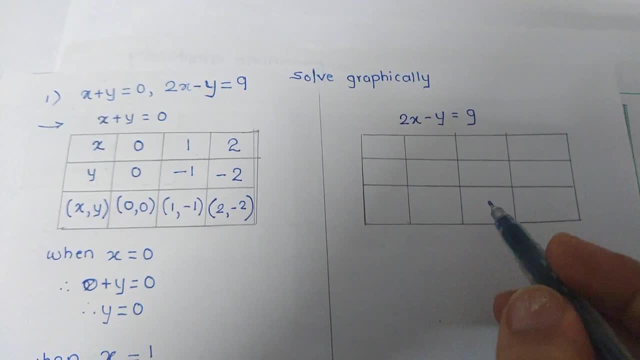 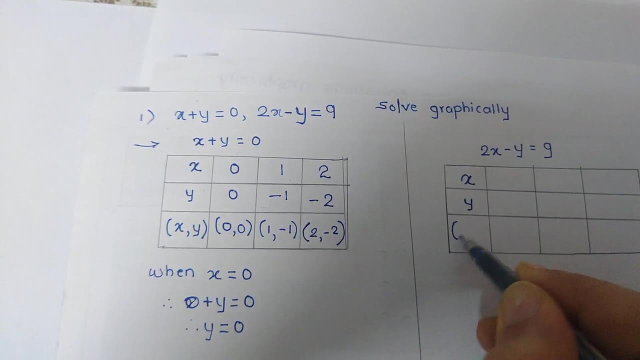 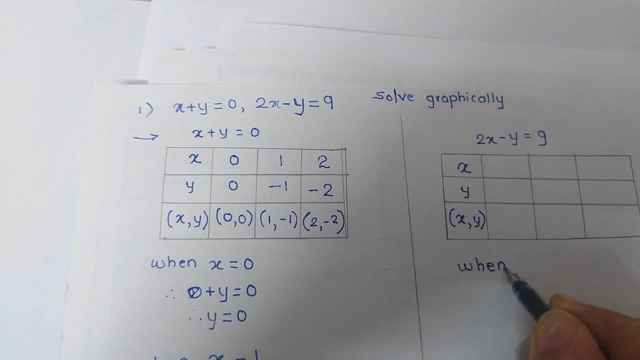 A table is prepared. Again, the table has 4 columns. In first column now you can write in first row x, y, and last row we can write in bracket x, y. So same like for first equation, we consider different values. 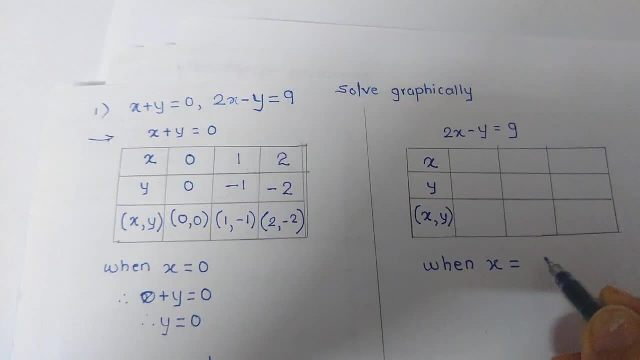 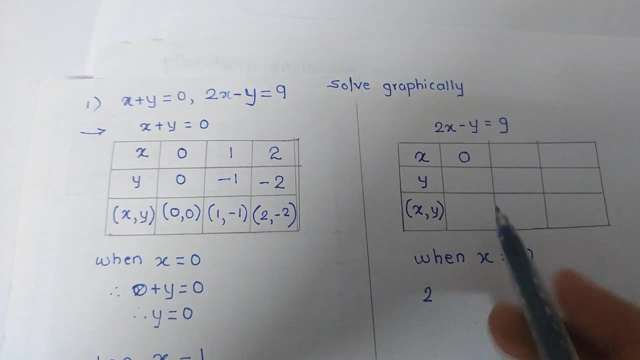 For x. when x is equal to, you can take any value. I start with 0.. So when x is 0, what will be value of y? For that we have to do the calculation. So the equation is 2x minus y, equal to 9.. 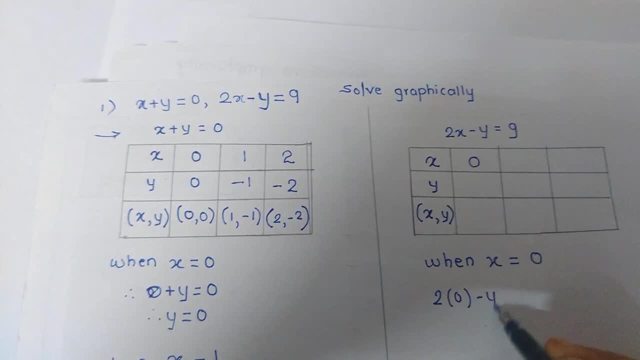 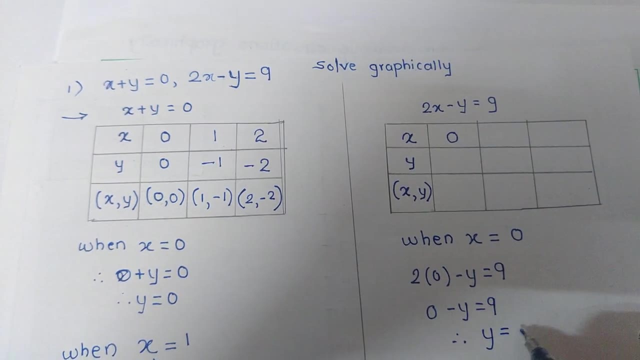 In place of x. I will write: the value of x minus y is equal to 9.. 2 into 0 is 0.. 0 minus y is 9.. Therefore y is minus 9.. It means when x is 0, value of y is minus 9.. 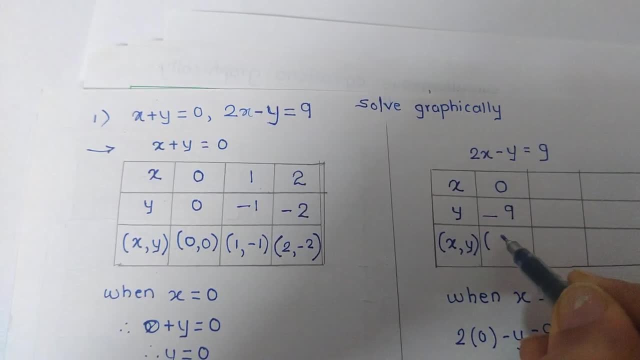 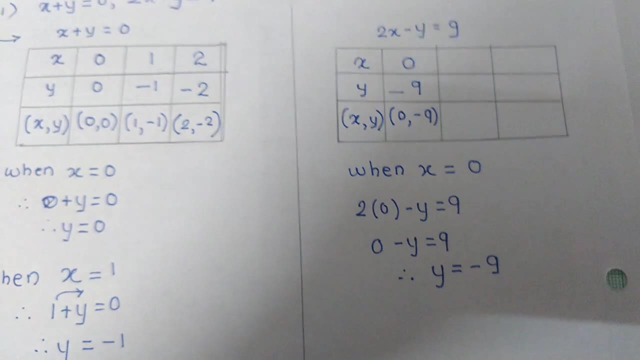 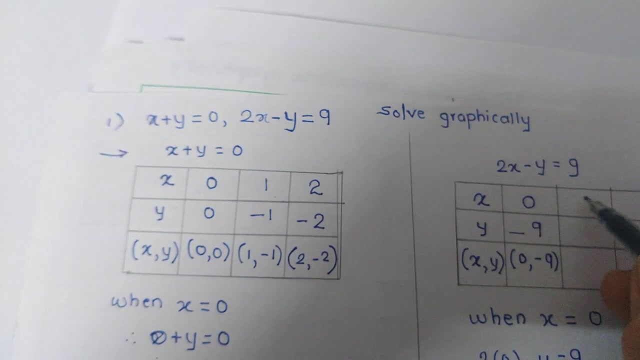 Let us write it So: the equation table, So the coordinate of the point is 0 minus 9.. 0 is x coordinate, minus 9 is y coordinate. Now for next value. when x is equal to next, I consider x is equal to 1.. 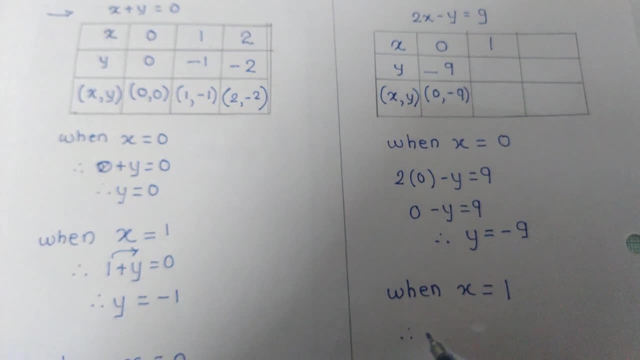 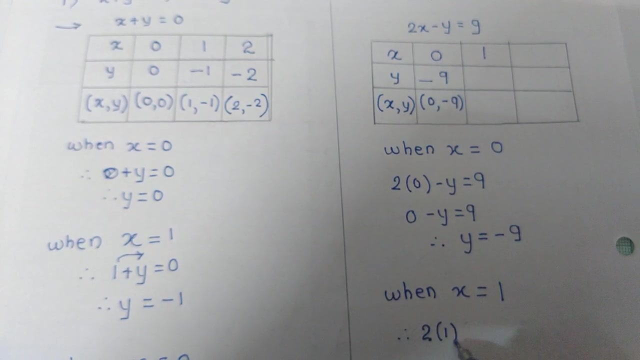 So when x is 1, value of y will be obtained by calculation. So equation is 2x minus y equal to 9.. In place of x I write value 1 minus y is 9.. So therefore, 2 minus y is 9.. 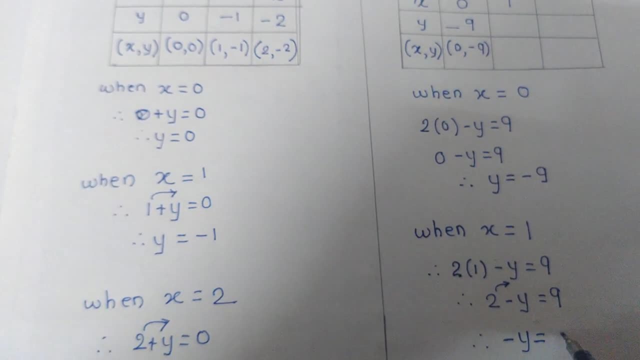 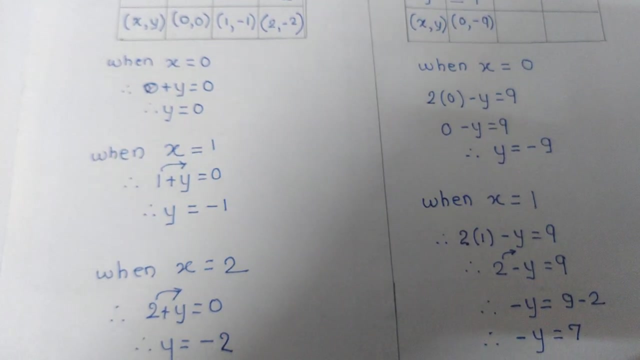 Therefore 2 will be transferred on other side of equal to. So minus y is equal to 9 minus 2.. Therefore minus y is 7. And therefore y is minus 7.. It means when you take x as 1, y will be minus 7.. 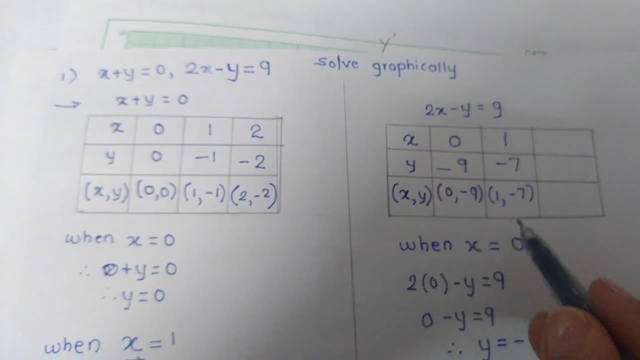 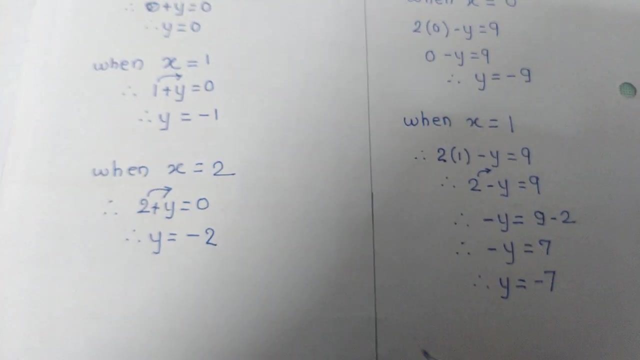 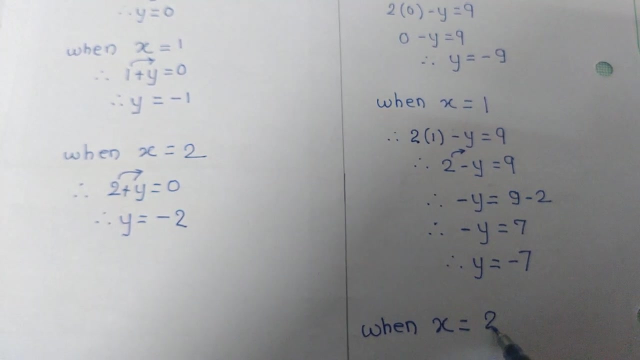 So you get the point 1 minus 7.. And be careful: always x coordinate is written first and then you write the y coordinate Next. for third value: when x is equal to randomly, you can consider any value, You can take any number. I take now x equal to 2.. 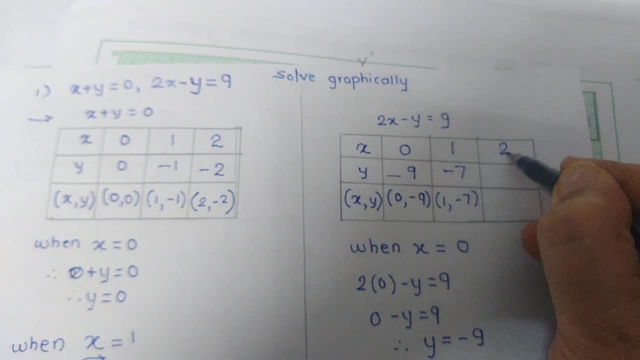 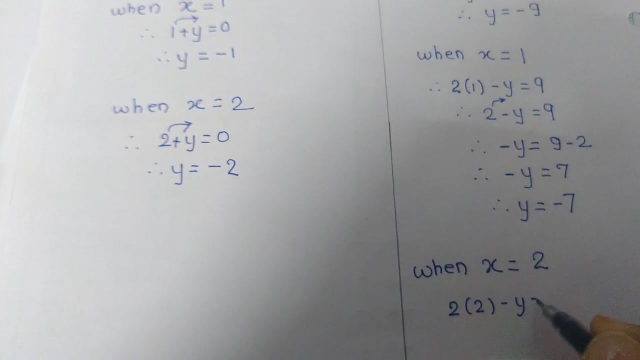 So when x is 2, we have to calculate the value of y. Equation is: 2x minus y is 9.. So 2 into 2 minus y is 9.. So therefore, 4 minus y is 9.. 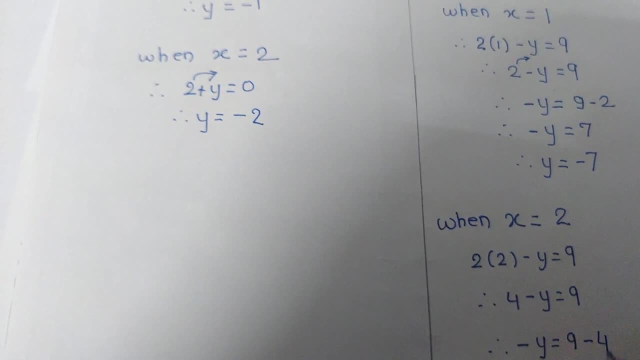 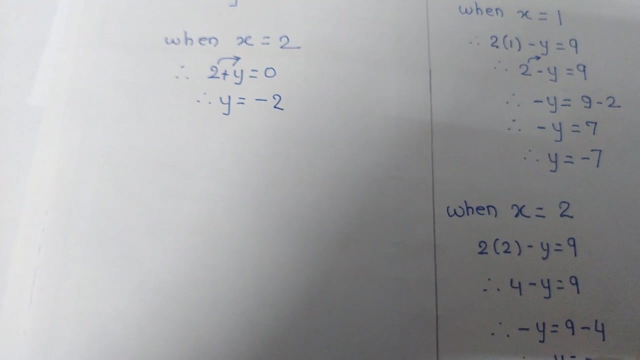 So therefore minus y is 9 minus 4.. 4 is 3.. Transferred on other side of equal to, So we have written minus 4.. Therefore, minus y is minus 5.. And value of y is sorry, not minus 5,. 9 minus 4 is 5.. 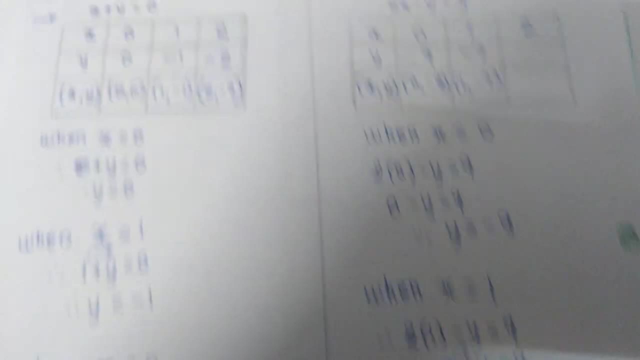 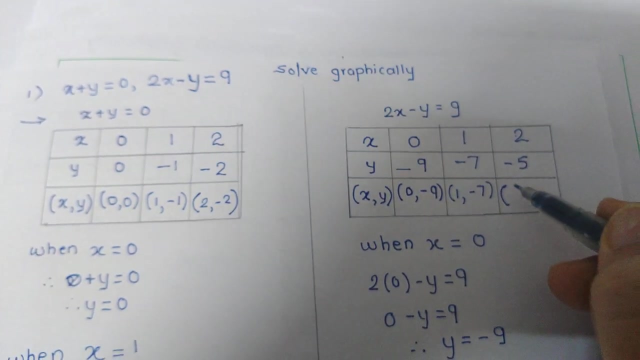 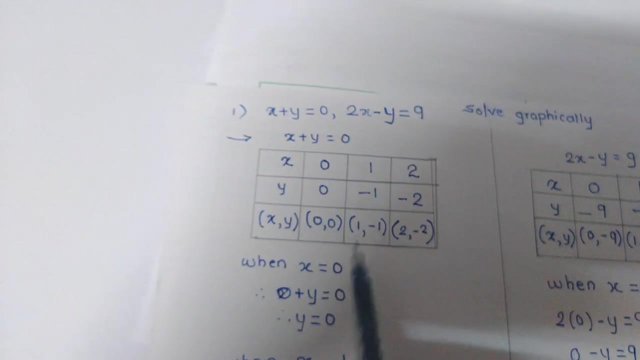 So value of y is minus 5.. So it means when you take x as 2, y is minus 5.. Point has coordinates 2 minus 5.. So in graphical method, what we have, What we have to do, is first we have to find 3 coordinates. 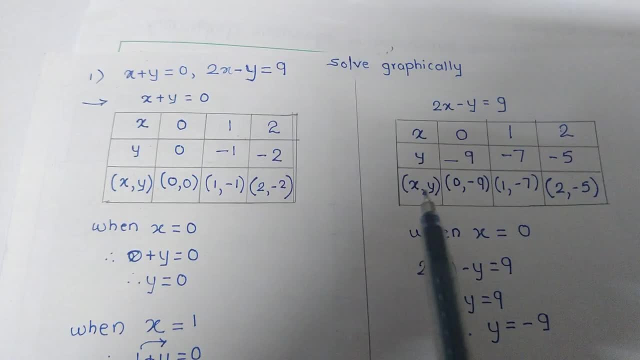 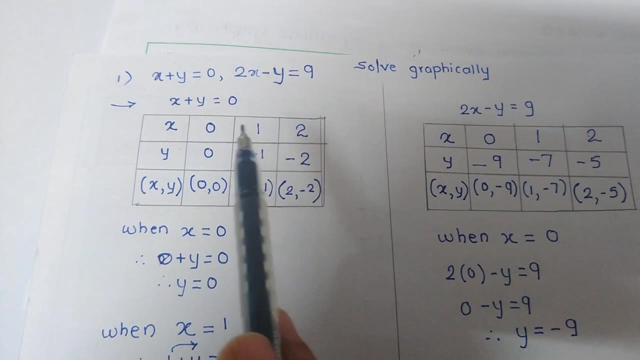 For one equation we have found 3 coordinates. For second equation also, we have found 3 coordinates. How to find coordinates? X values you can consider on your own Any value you can take, either positive, negative or 0. And y value you obtain by calculation. 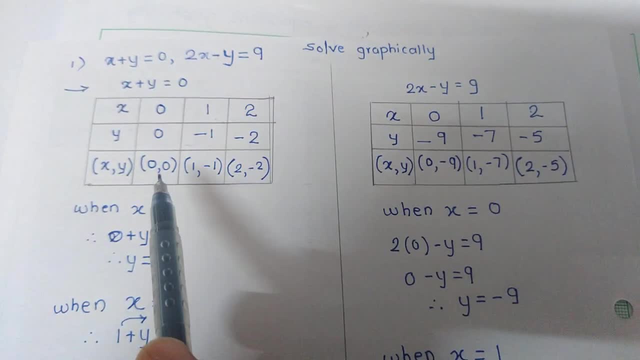 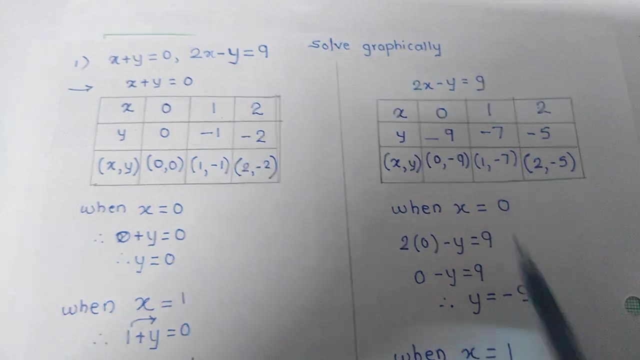 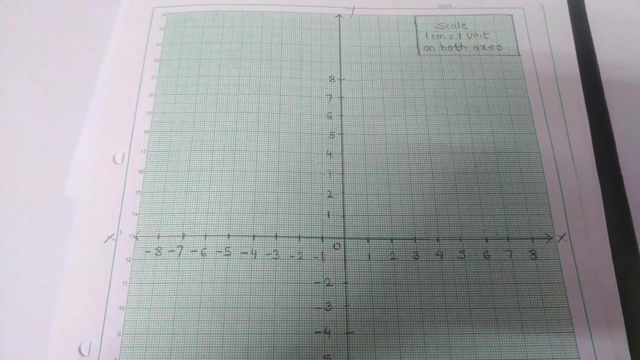 Similarly same step we have done for the second equation. Now we have got 3 points for first equation and 3 points for second equation. These 3 points we have to plot on a graph. Now take a graph paper. On a graph paper, draw a vertical line and horizontal line representing x-axis and y-axis. 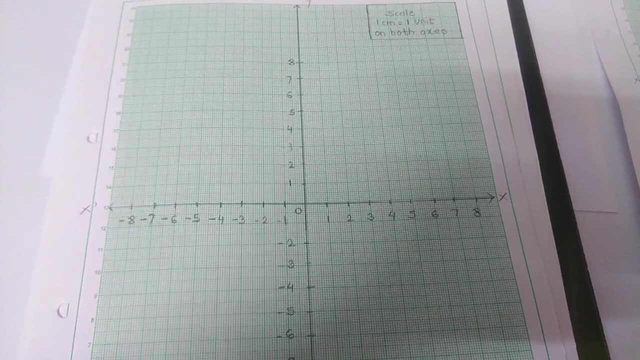 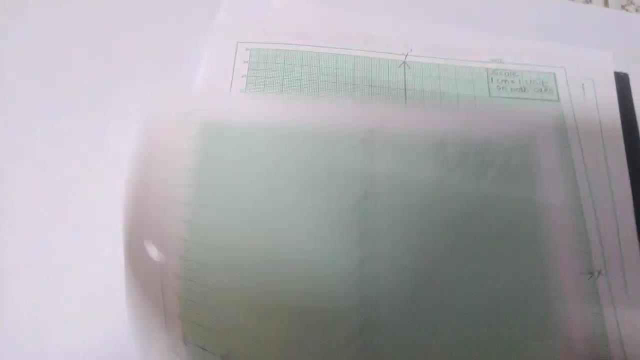 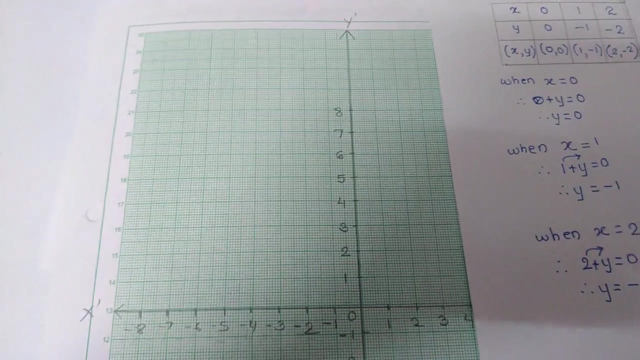 And now what we have to do is the coordinates, the points which we have got on calculation, we have to represent on graph. So the first point of our calculation is first point is 0, 0.. So let's plot this point: 0, 0.. 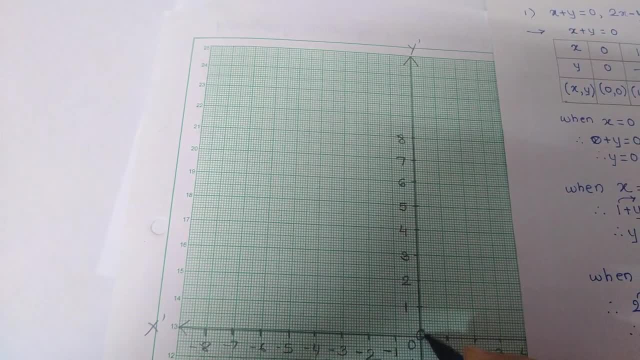 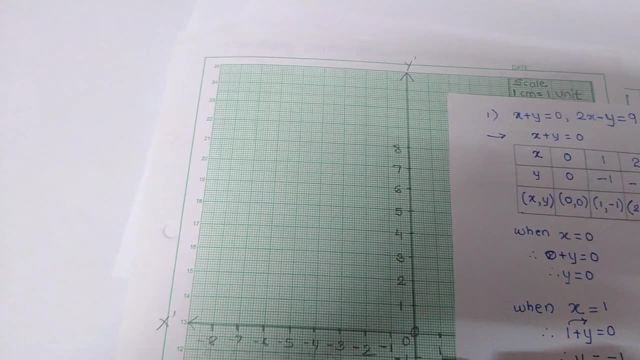 So x is 0.. So y is 0.. This is the point. Second point of calculation is 1, minus 1.. So 1 is x coordinate minus 1 is y coordinate. This is the point. 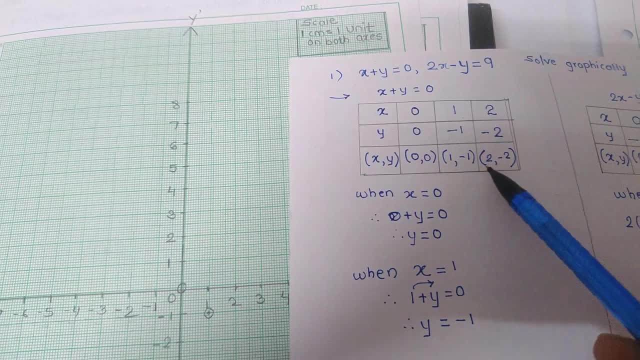 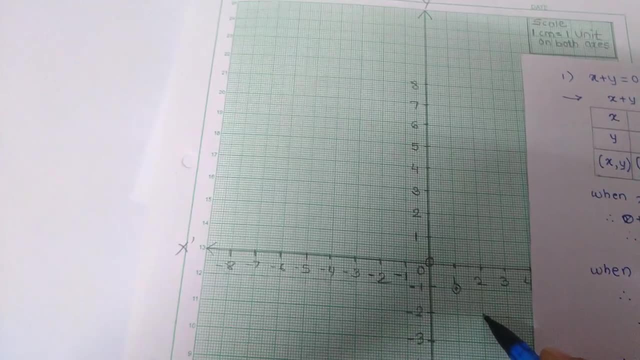 Next point of our calculation is 2, minus 2.. First coordinate is x coordinate. Second coordinate is y coordinate. So this is 2 and minus 2.. This is the point. This is for first line. After getting the 3 points, with the help of scale, join these 3 points. 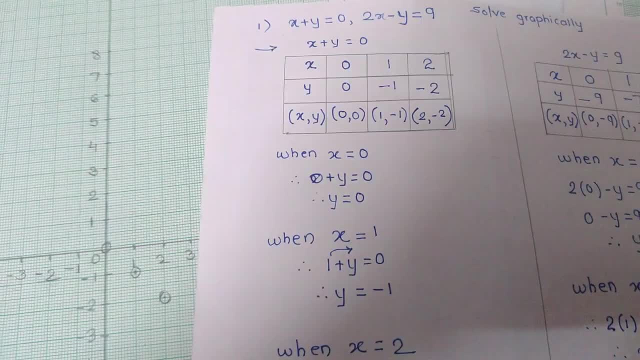 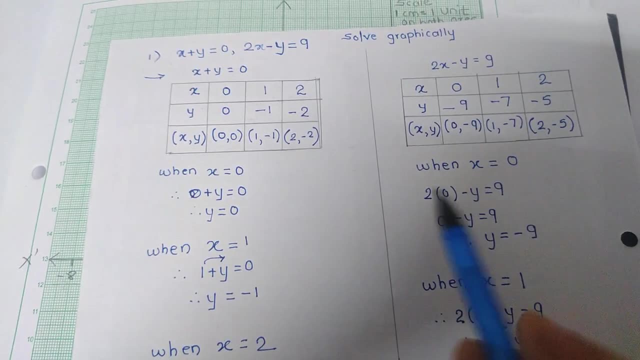 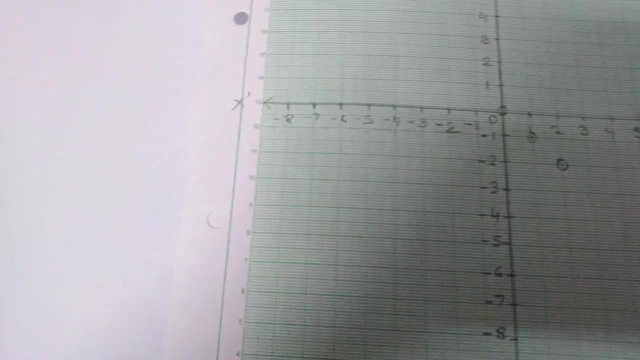 And get a straight line. Similarly, we will plot the points for second line, which is 0, minus 9.. 0, minus 9.. Now x coordinate is 0.. Y coordinate is minus 9.. As x coordinate is 0,, the point will lie on y coordinate. 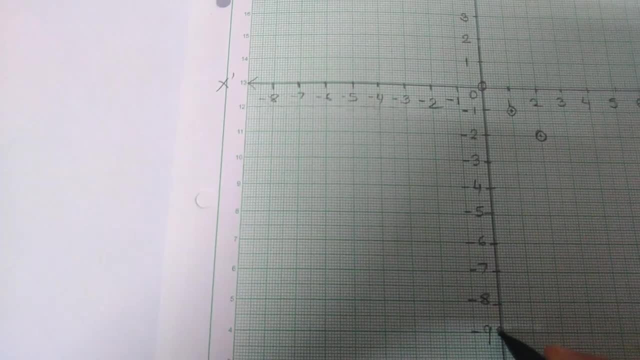 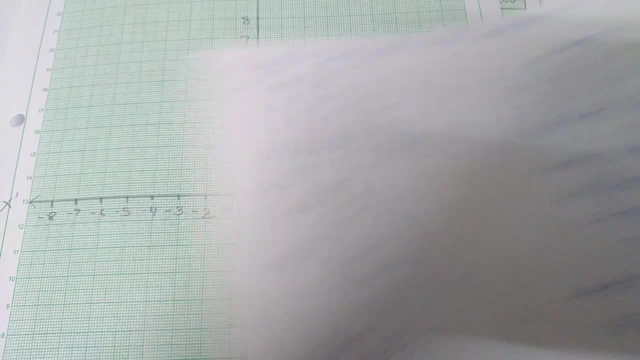 So here is the point: minus 9.. Second point is 1, minus 7.. x coordinate is 1.. Y coordinate is minus 7.. So the point x is 1.. y is minus 7.. This is the point. 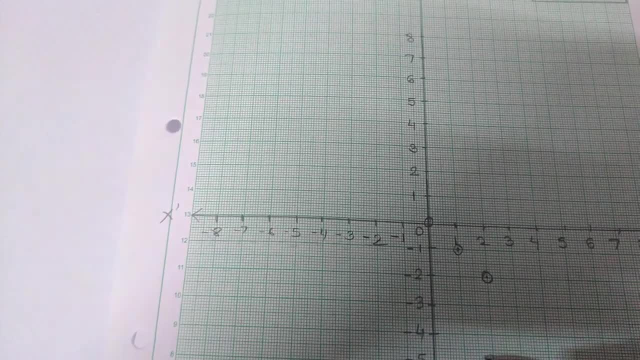 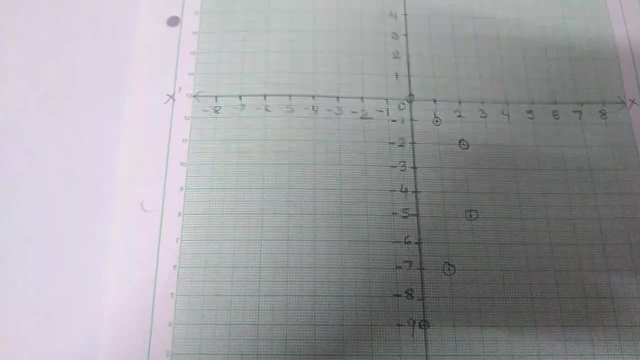 Last point is 2, minus 5.. x coordinate is 2.. y coordinate is minus 5.. We have got 3 points. By joining these 3 points we will get line, And the point of intersection of 2 lines is the solution of equation. 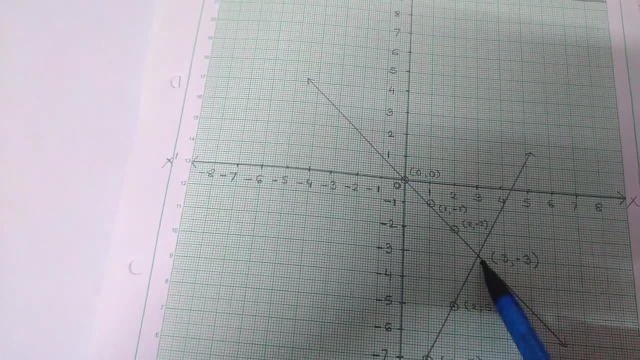 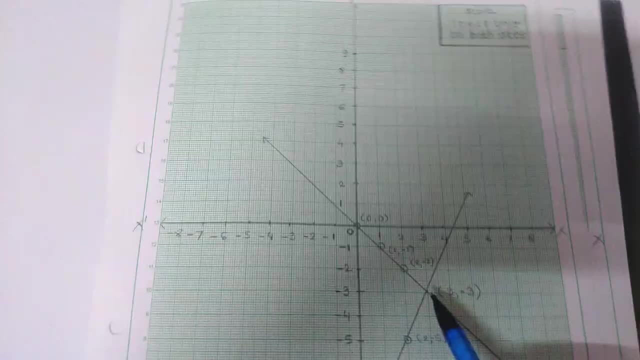 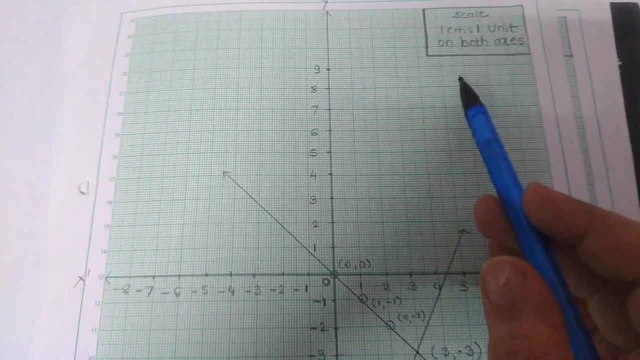 So, after joining both the lines, both lines intersect at point 3, minus 3.. So 3, minus 3 is solution of equation. Always remember on a graph paper, when you draw axis, don't forget to label y, y, dash, x, x, dash. write the scale on a graph paper.